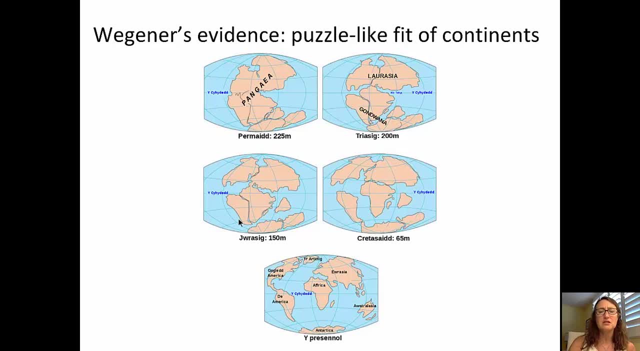 Moving back a little further in time, 150 years ago, you see the big one which is the puzzle-like fit of South America and Africa together here, And we can continue back in time to when Pangea would have been one single supercontinent. 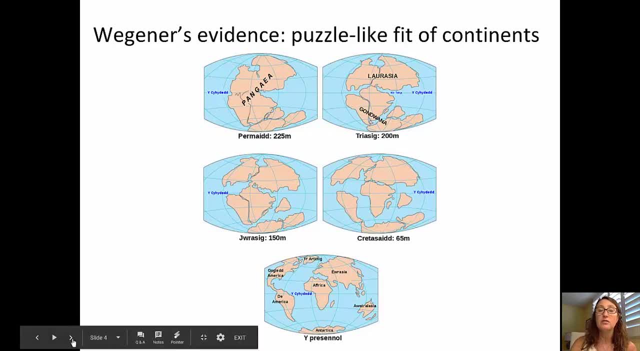 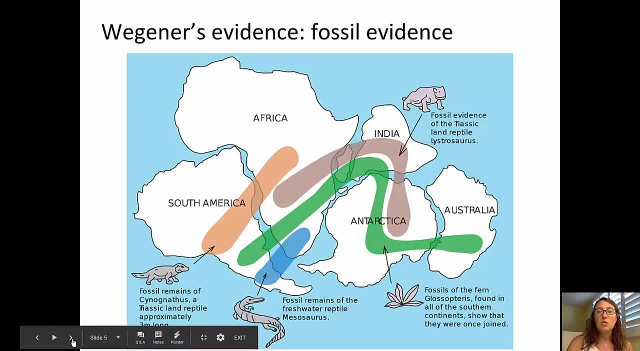 So this is the puzzle-like fit that Alfred Wagner was pointing to as one of the prime pieces of evidence for his theory of continental drift. Another piece of evidence was that Wagner had fossil evidence for several different species that helped support his idea that continents had fit together into one supercontinent. 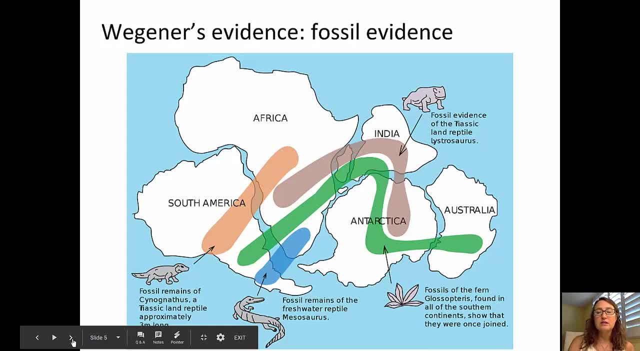 Pangea in the past. So in this diagram you can see that there is fossil evidence for this reptile from the Triassic time period called Lystrosaurus, And fossils of Lystrosaurus have been found In Antarctica- yes, Antarctica, a reptile in India and over into Africa. 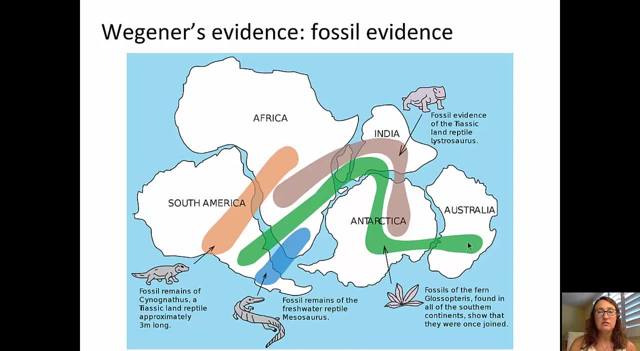 Also, a plant fossil named Glossopteris is found across Australia, Antarctica again, India, Africa and into South America. Another fossil, Mesosaurus, a freshwater reptile, found in Southern Africa and Southern South America. And a fourth fossil, Cynognathus, who was found across South Africa. 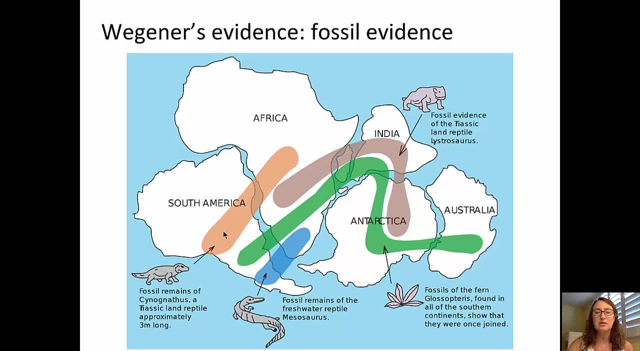 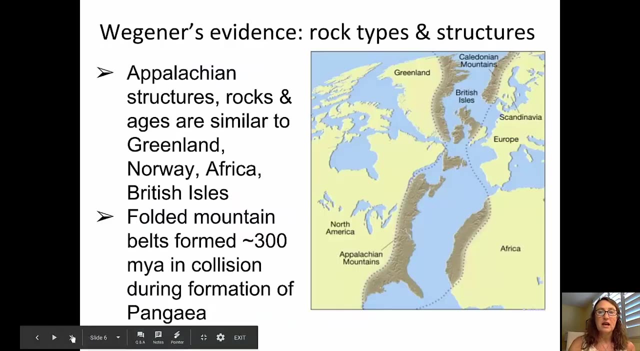 America and Africa. So if you look at the patterns there, it's easy to believe that if those continents had been attached, those creatures or that plant might have been evolving at the same time across those landmasses as they were attached to one another. An additional piece of evidence. 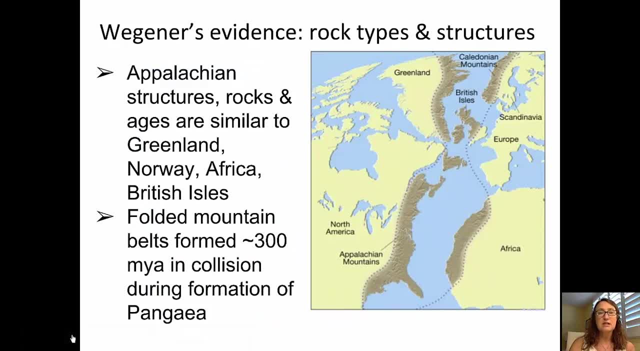 that Wegener pointed to was that there are rock structures and rock types and ages that are similar on either side of the Atlantic Ocean. So here you can see in the brown color the Caledonian Mountains up here in Scandinavia. the same rocks, structures and ages found in the British Isles found along